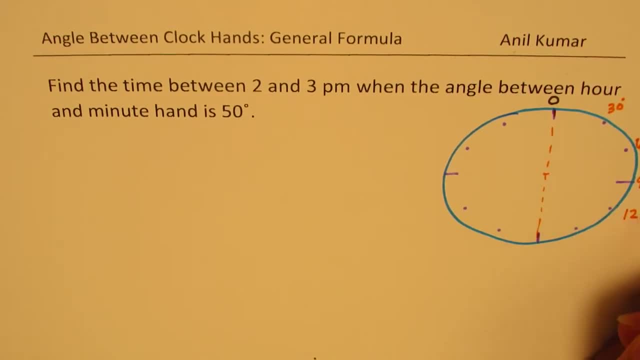 60. 90., 120. 150., 180. And so on. right, So that is how the angles are. So within every hour there is 30 minutes. Now we are saying: find the time between 2 to 3 hours. That means we want. 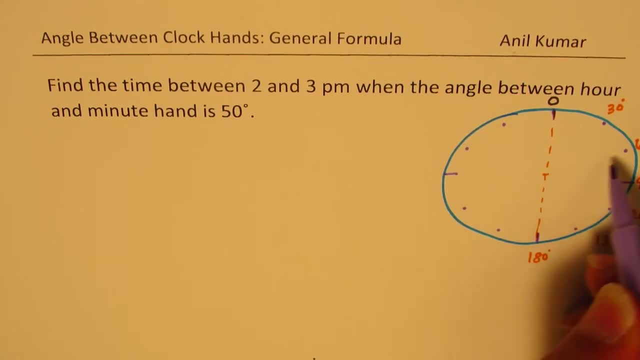 a situation where the hour hand is somewhere between these two and the minute hand is 50 degrees away. To say that our hand, let's say is, let's say here, for example: right, Let's say, our hand is here, In that case minute's hand is 50 away. So 50 away means 2 hours, 60, right So? 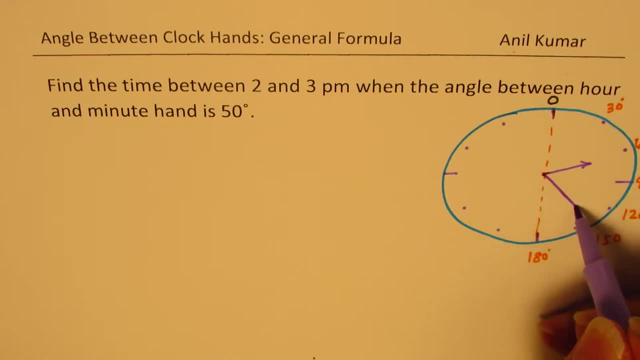 somewhere, somewhere like this, Do you understand? So we exactly don't know where, but somewhere like this, correct, Right. So we need to find this position. We don't know what this position is, but that angle should be 50 degrees. That's what we need, correct? Well, one more situation could be that this arm is on. 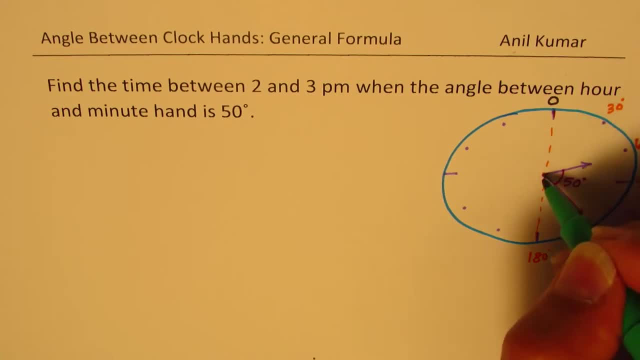 the other side right. So that is to say, we could also have this somewhere here right And somewhere there some some position between 2 to 3. And we could also have an angle of 50 degrees. So that's. 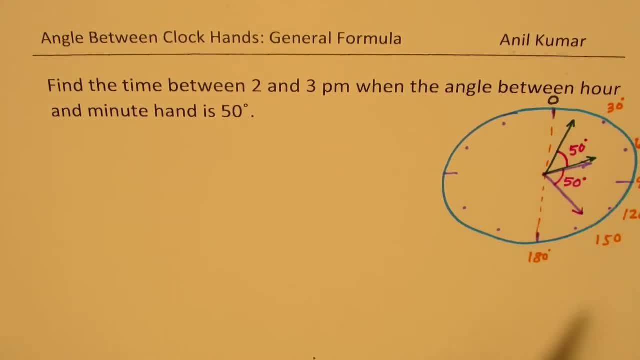 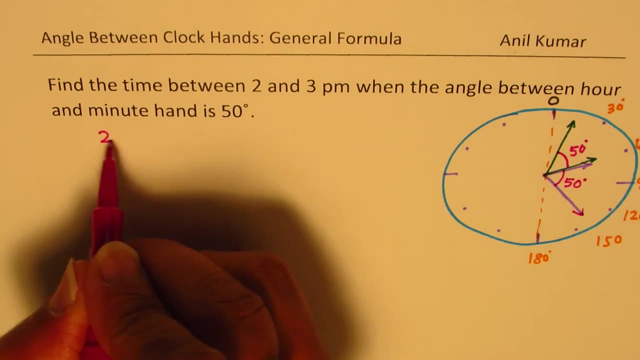 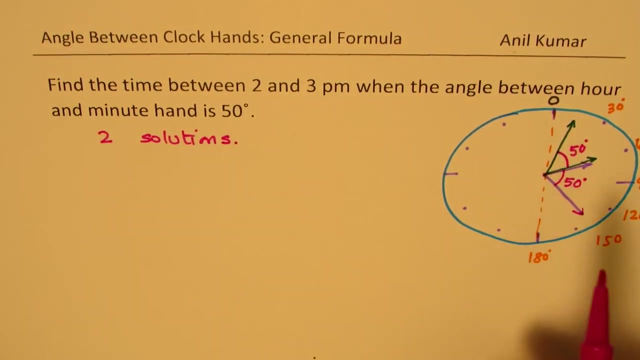 50 degrees between the two Right. So when we say that the angle is 50 degrees, we are actually looking for two solutions. So in one case, the hour hand is beyond the minute's hand. The other case, minute's hand is beyond the hour hand. You get an idea, correct? 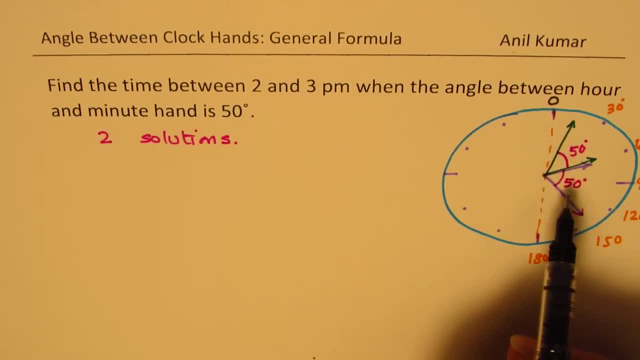 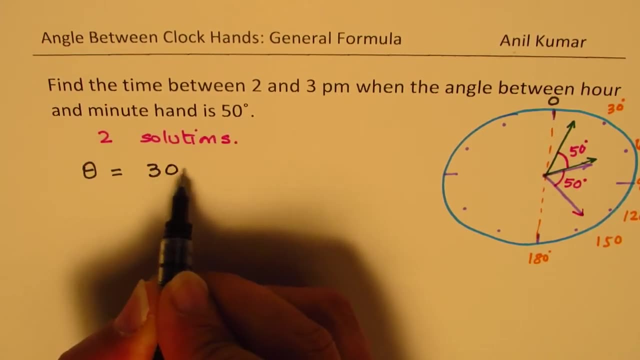 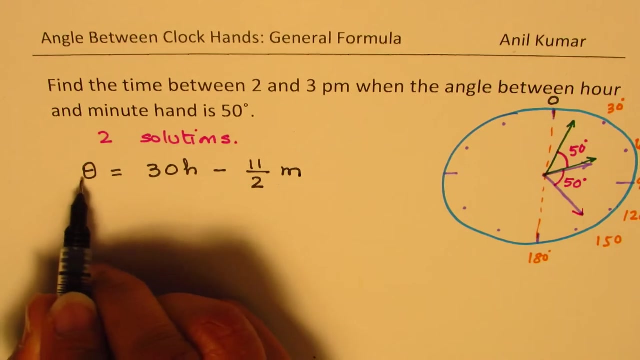 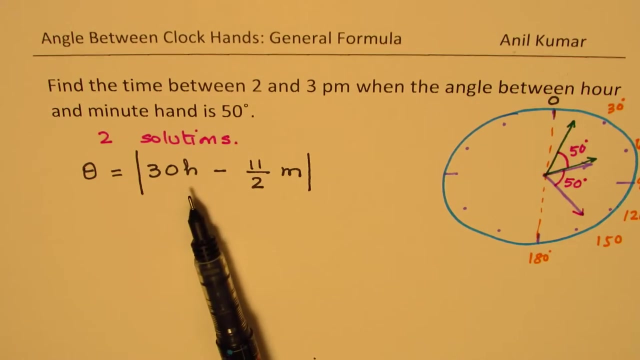 We also know from the speed of hour and the minute's hand that the angle can be given by the formula theta equals to 30 times h minus 11 by 2 times the minutes, And this angle is always positive. So we take a positive value. That is the absolute value of this right. So in our case we for sure know that. 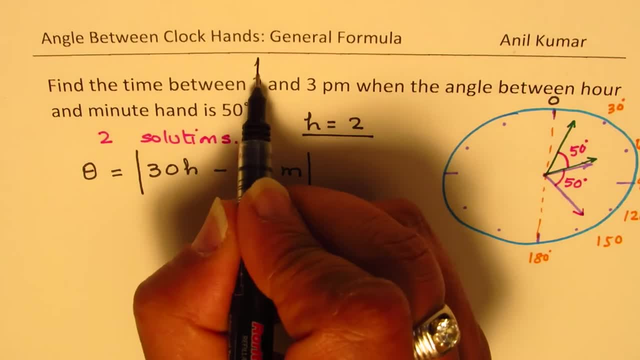 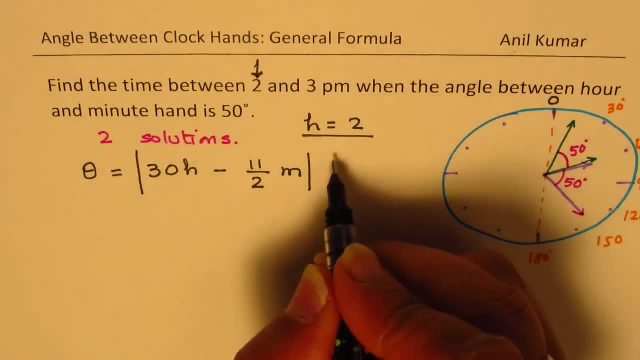 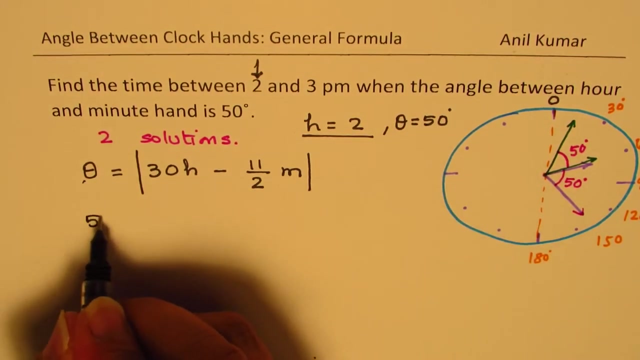 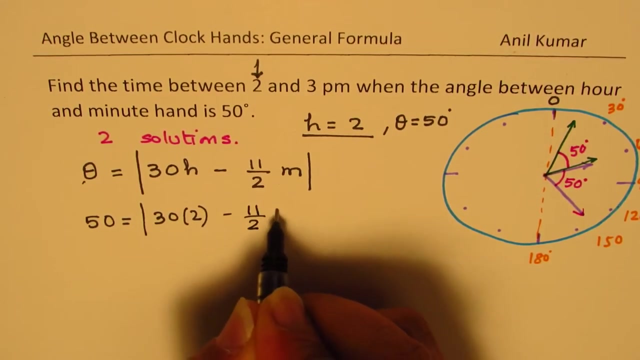 h is 2.. H is 2 hours between 2.. So we will start somewhere. more than 2, right, But less than 3.. So h is 2.. We also know that theta is 50 degrees. Using this formula we can write down: 50 equals to absolute value of 30 times 2 minus 11 over 2 minutes, And then we can find the minutes. 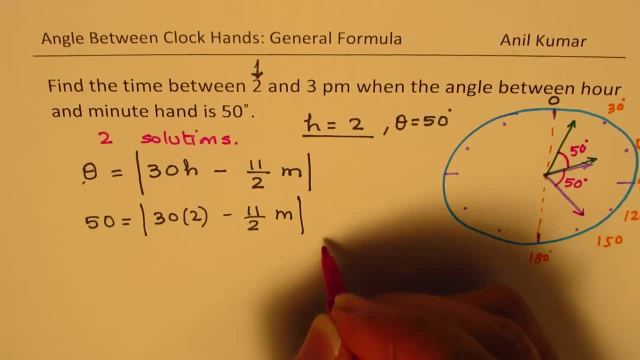 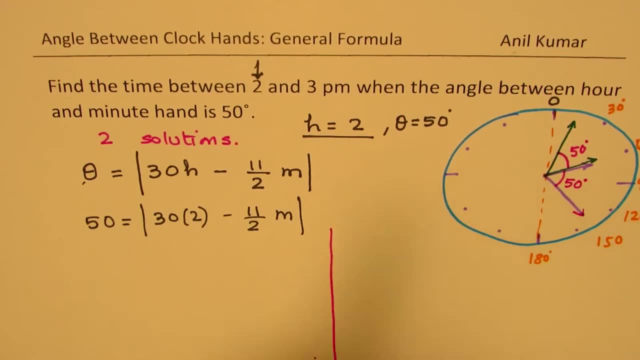 Absolute value basically means that we could solve for two equations. All this inside could be either positive 50 or negative 50. But absolute value will be positive. You get the idea right. So we could write this as: 30 times 2 is 60. 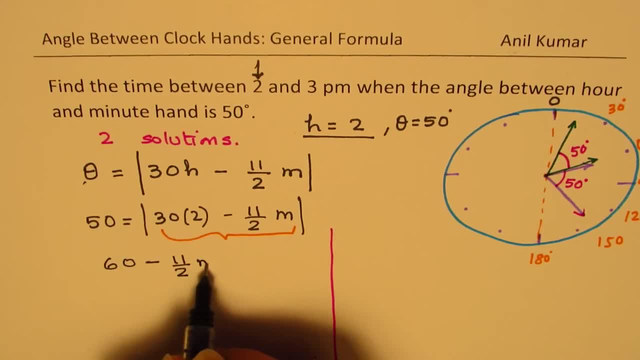 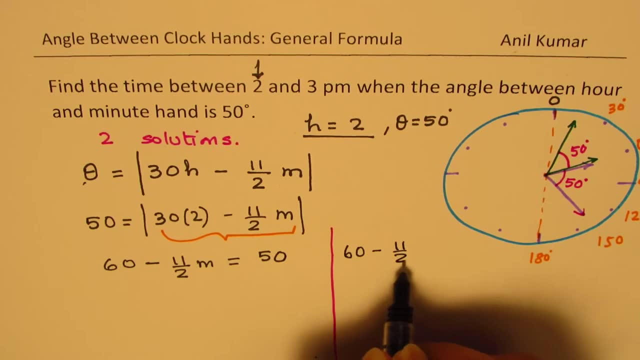 minus half of 2m equals to positive 50. Or this could also be 60 minus 11 by 2 and equals to minus 50, clear, Because absolute value of minus 50 is also 50. You get the idea right. 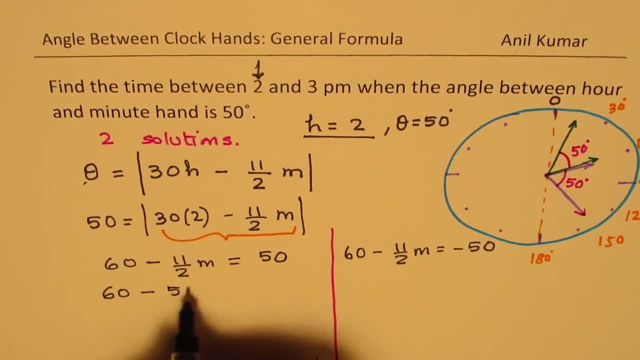 So, taking this to the right side, we get 60 minus 50 equals to 11 by 2m and that is 10, and then we'll multiply by 2 over 11 to get the value of m correct. So that is 20 by 11, which is 1 and 11. when you take away, you get 9 over 11 minutes, correct. 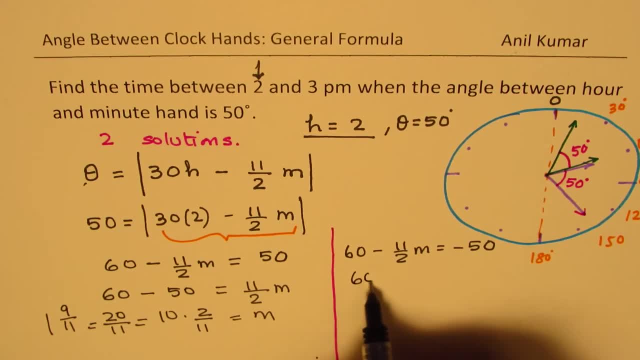 On this side we have 60 plus 50 equals to 11 over 2m, or we have 110 times 2 over 11 equals to m, and that gives you m equals to. this goes: 10 times m equals to 20, right. 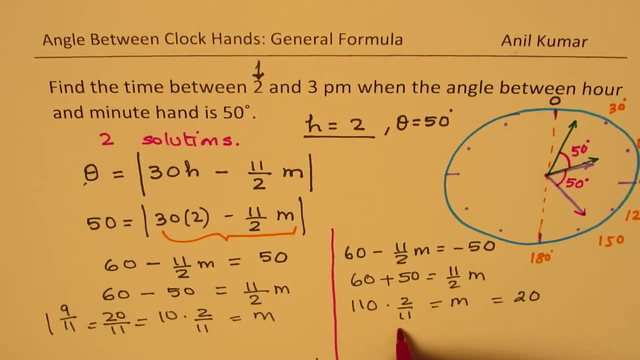 So we have two solutions here. One of the time could be 220, right? The other will be 2, 1, 9 by 11 minutes, right? So slightly very close to 2 minutes, right? So basically, I should write 2 hours and so many minutes, right? 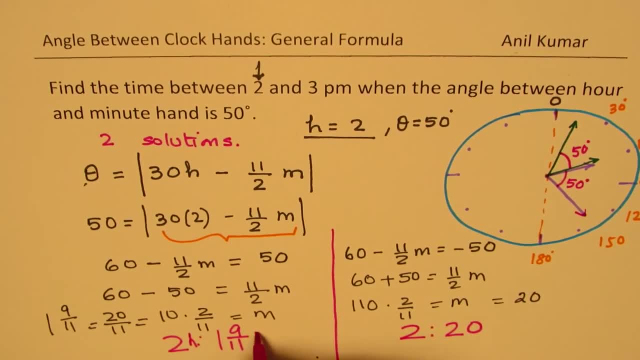 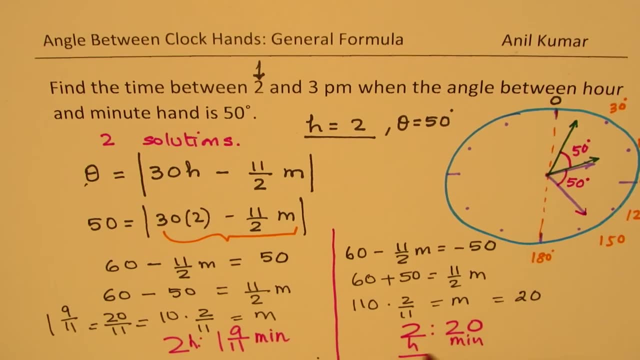 So many minutes, 2 hours. I should write 2 hours and so many minutes. is that clear? So it is 2 hours and 20 minutes in this case, correct? So that is How you could actually solve this equation. 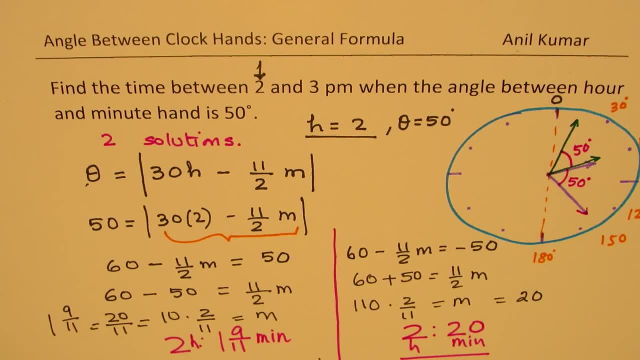 So that should be, I think, clear and straightforward. Now to look into this, I'll provide you with a link for the derivation of this formula. How do we get this formula as the angle theta being equal to 30 times hours minus 11 by 2 times minutes? perfect. 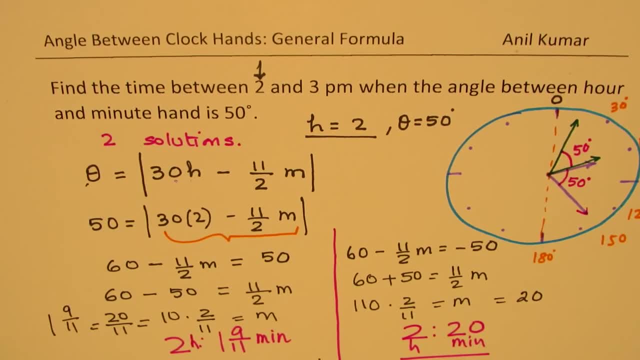 But I hope that helps you to understand that the idea here is to find two different solutions- Right, Since the minutes could be before hours or after hours are- and then solve it. Hope it makes sense. Feel free to write your comment, share your views and, if you like, and subscribe to my 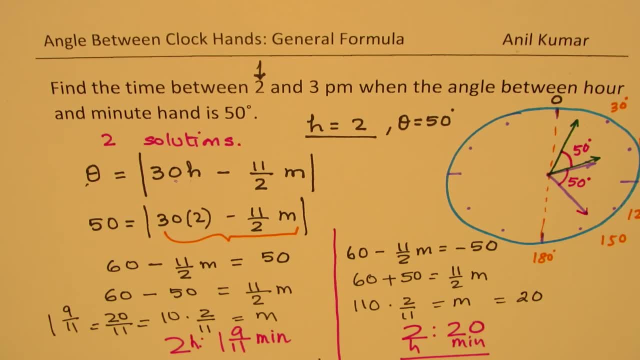 videos. that'd be great. Thanks for watching and all the best. 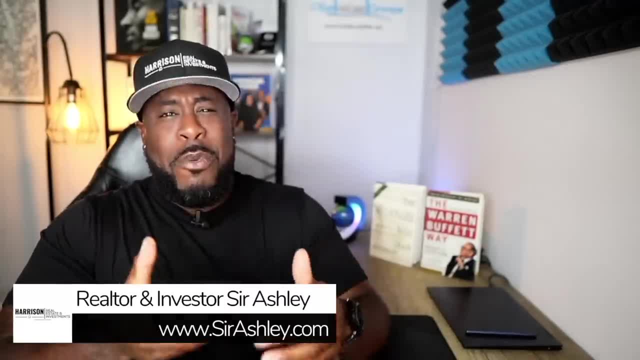 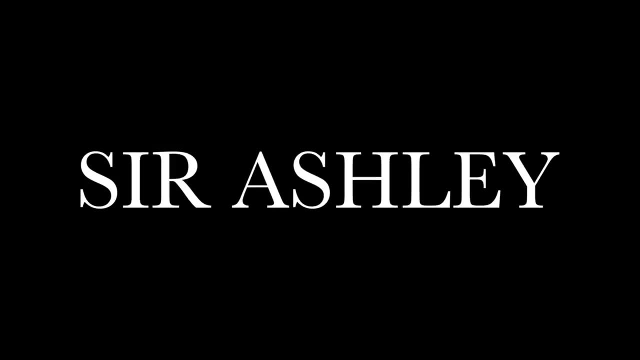 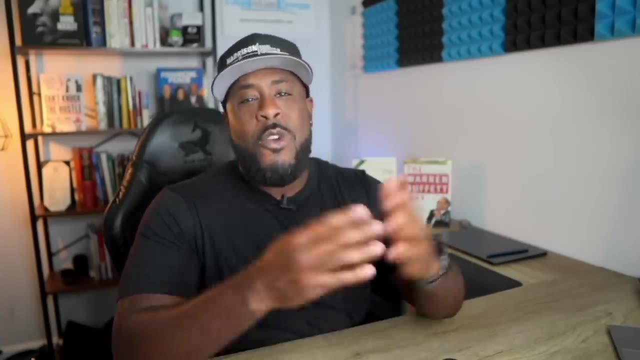 North Carolina can be a wonderful place to live, but today I'm going to give you about 10 reasons why you might want to avoid this place. Stick around, Hello, family. My name is Sir Ashley. I'm a realtor and investor in North and South Carolina. 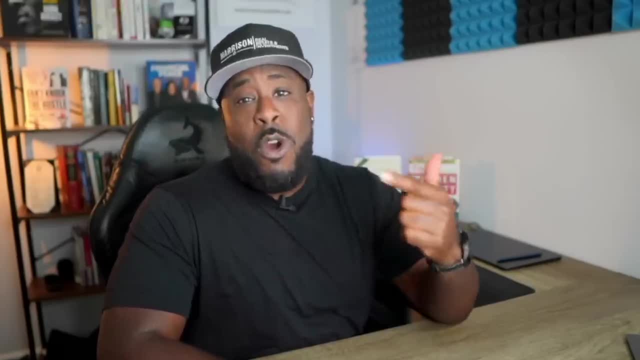 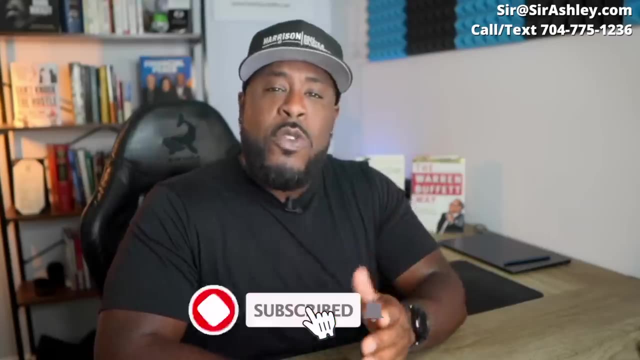 And if you're interested in learning what it's like to live, work, play, eat, buy real estate in either North or South Carolina, this is the channel for you. So make sure you hit that subscribe button and tap on that bell icon so you can be alerted when we come out with a new video. 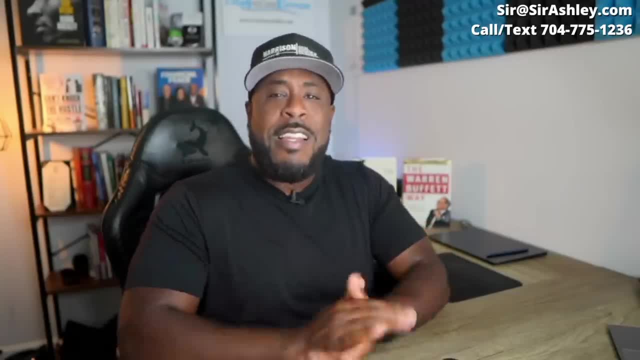 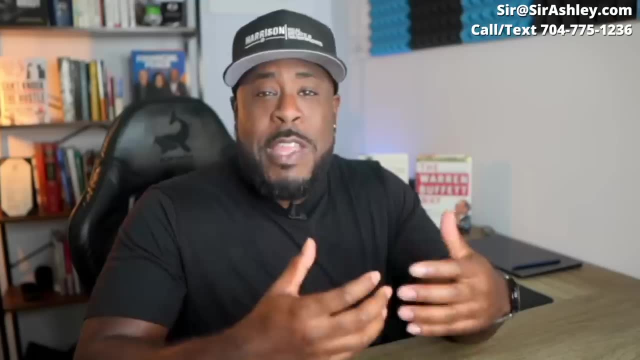 So I have many people reaching out asking me what is it like living in North Carolina and what can they expect? And I absolutely love it And my team and I love giving you feedback and just having a dialogue with all of you that reach out. So if that is you and you have any questions, 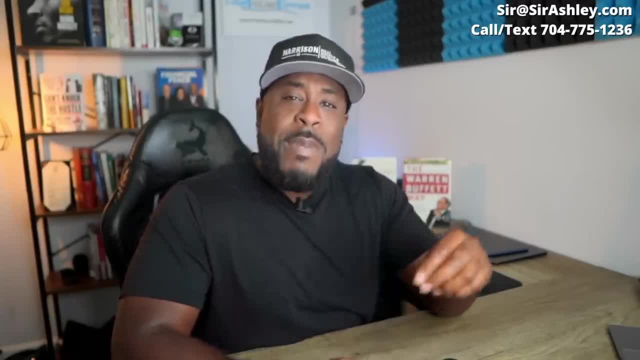 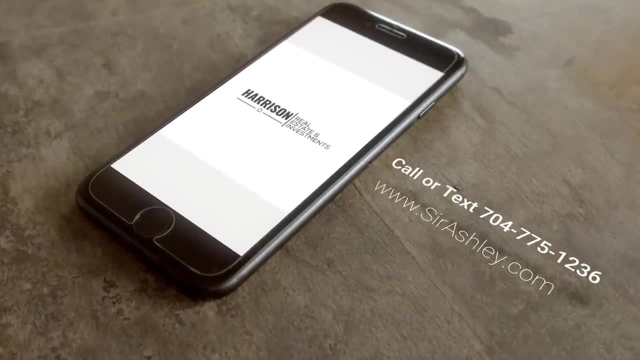 about what it's like living here. make sure you leave a comment after this video or you can reach out to us, whether it be a phone call, a text or an email, And I'll see you in the next video. Now I personally love talking to people about what it's like relocating to North Carolina.